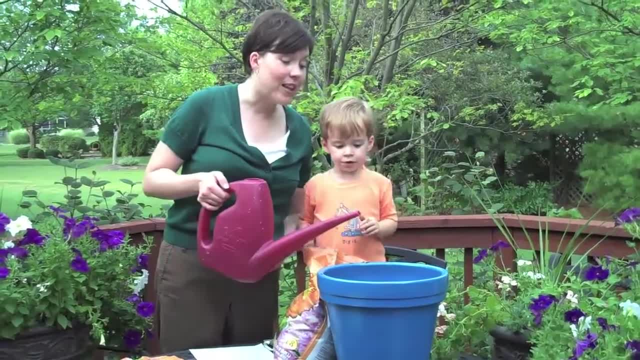 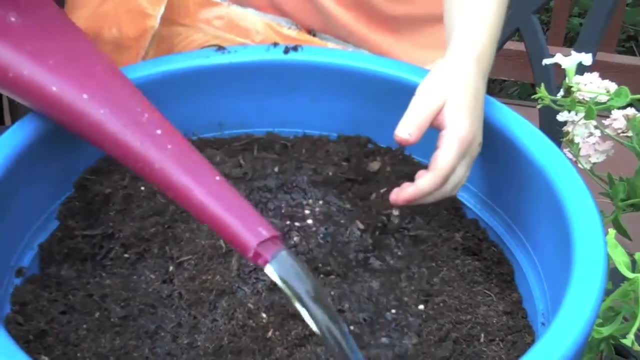 more. Yeah, that's perfect. Okay, Now water your lettuce with cold water. You want to make sure that the soil is dry. Lettuce grows best in cooler temperatures, so if it's in the heat of the summer, try to find a shadier spot for your pot and make sure you keep your lettuce watered. 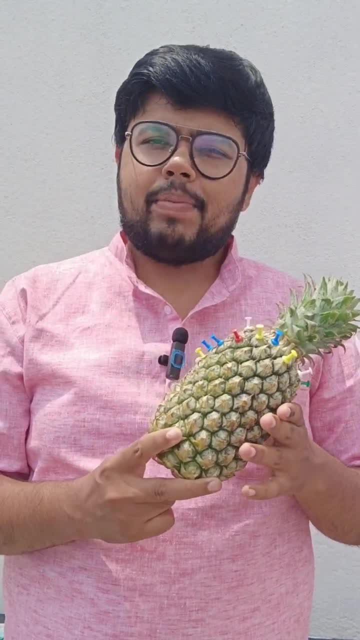 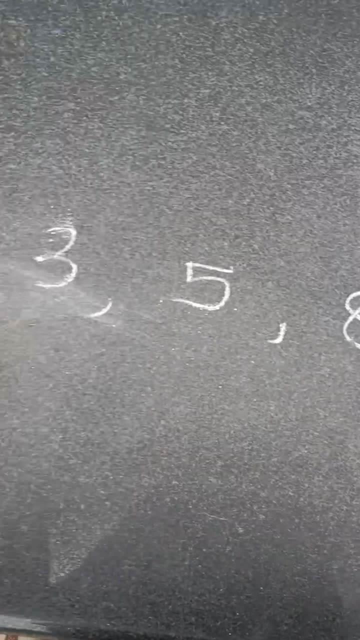 So this is a pineapple and there is a very interesting mathematics in this pineapple, So that is called as the Fibonacci series. So before going into this, let us first understand what is Fibonacci series. It's an interesting pattern. The pattern is: if you just add 1 plus 1. 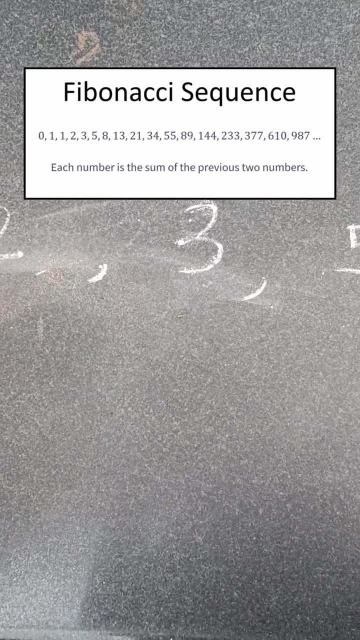 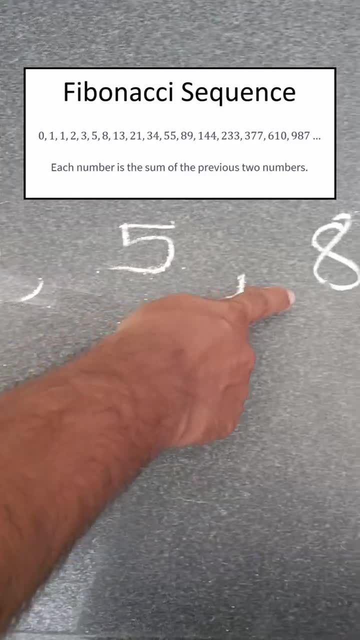 it is 2.. If you want this, 3,, 3 is the addition of the previous two numbers, 1 plus 2.. Next number, if you see it is the addition of the next the behind two numbers, 2 plus 3, 5. 8 is an addition. 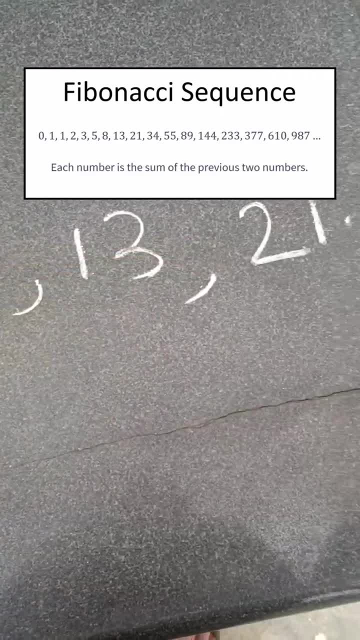 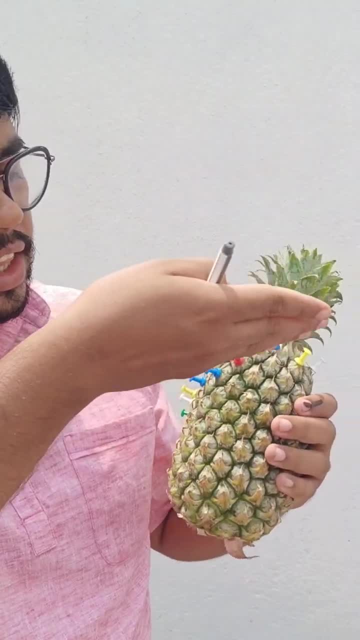 of previous two numbers, 3 plus 5, 8.. Same way it goes on, and this is called as the Fibonacci series. This is a pattern in this pineapple, So here already I have pinned. Okay, here you can see the spirals going in this manner and spirals going also in this manner. Okay, now we will just 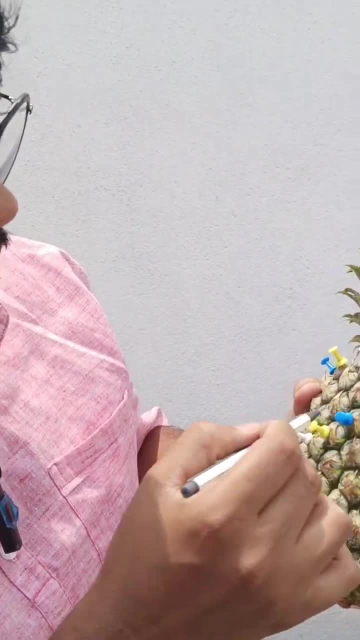 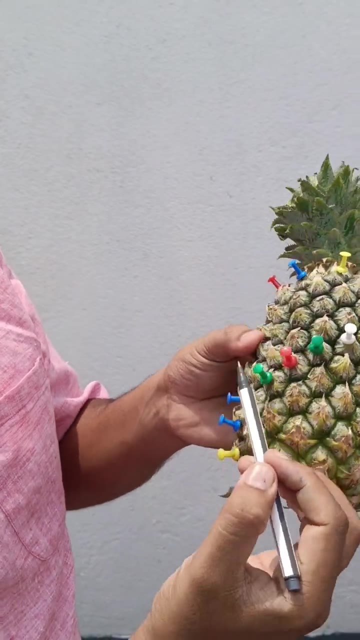 we will first see if you see the spirals going in. the spirals are going in this manner here. Count this: how many spirals? 1, 2, 3, 4, 5, 6, 7,, 8,, 9, 10,, 11,, 12, 13.. You can see there are 13. 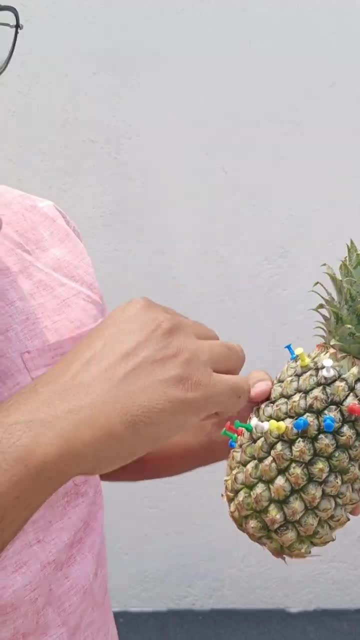 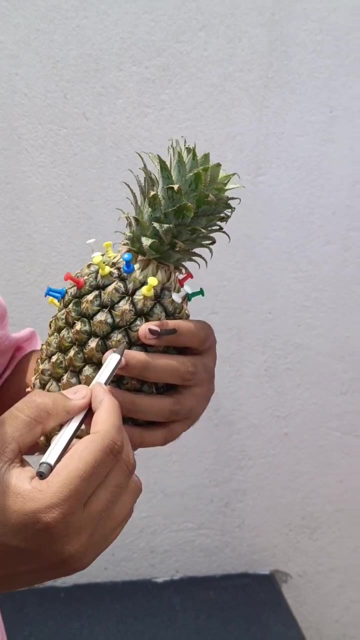 spirals here. Okay, it is again a Fibonacci series. Now we will count this manner. Okay, so I will just start 1.. I will just start with this blue color: 1,, 2,, 3, 4.. Okay, here you can see 5,, 6,, 7 and 8.. 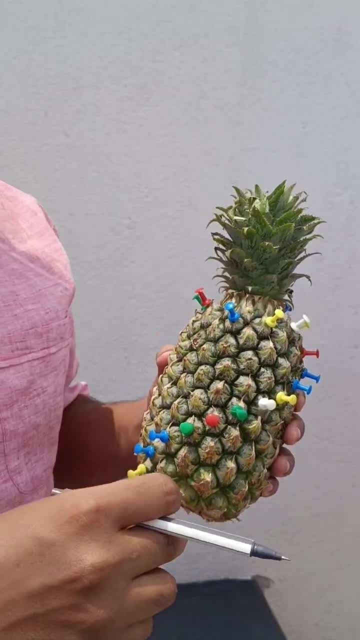 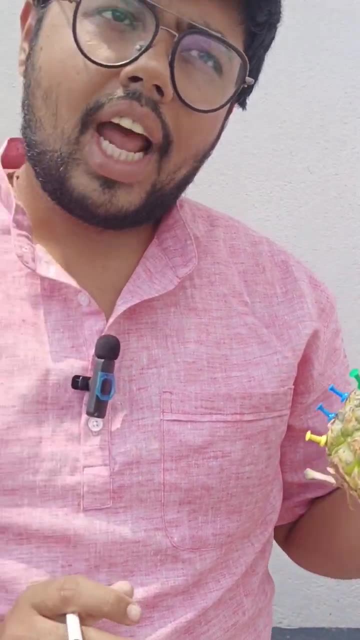 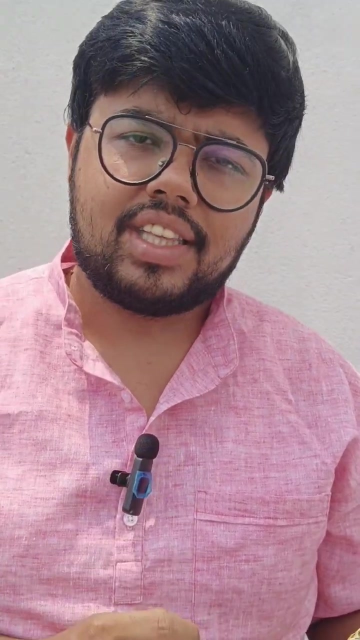 I started with the blue, so there are 8 in this manner, opposite manner. So 8 is also a Fibonacci series. So generally, if it a fully grown Fibonacci series is there in nature, that will help the to form absorption of sunlight And there is lot of science behind it. but this is a basic thing.